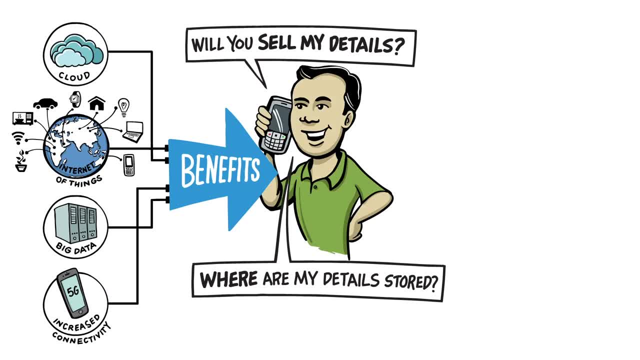 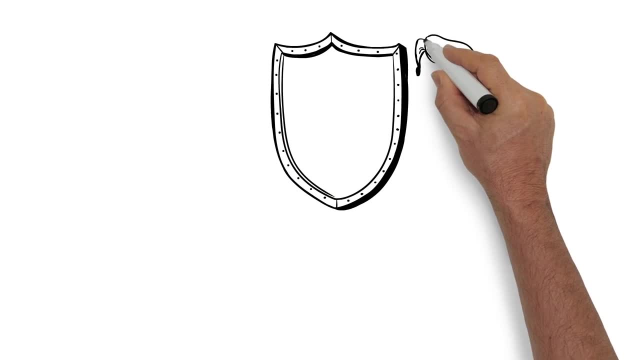 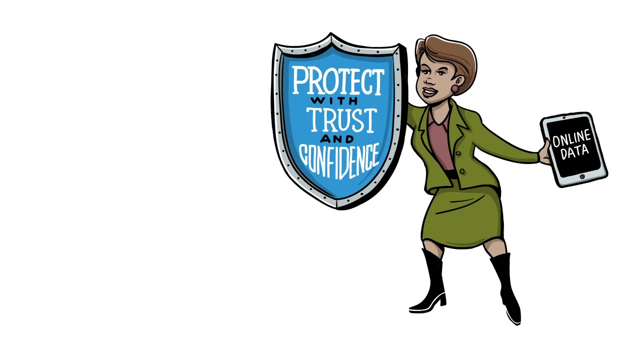 But they also make it more urgent to address various concerns over data and privacy. The challenge for data protection regimes is in managing the risks and addressing the concerns without restricting or eliminating the potential risks. The role of governments and the industry in protecting online data is of paramount importance. It must be done with a great deal of trust and confidence. 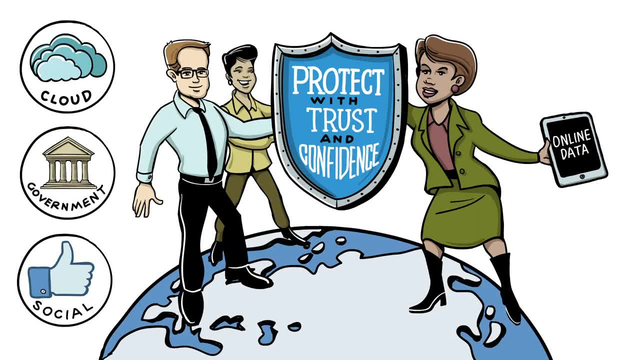 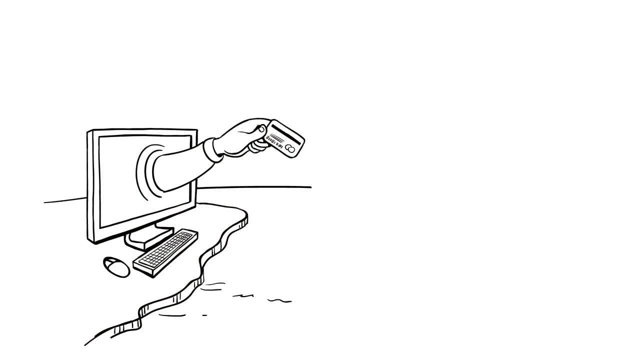 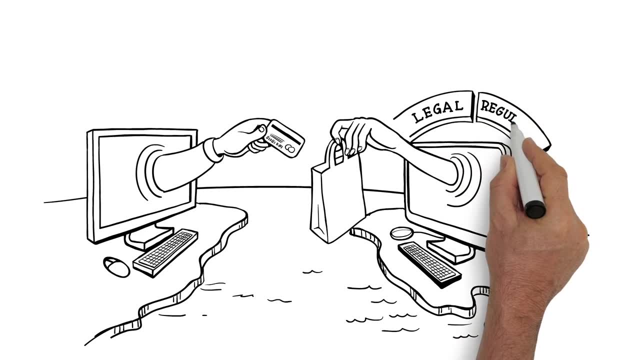 This requires collaboration across stakeholders and geographies. Cross-border e-commerce presents developing countries with amazing opportunities, but those countries that want to participate in the digital economy must consider the need for legal and regulatory support. They need regulatory frameworks to protect the personal data they collect. 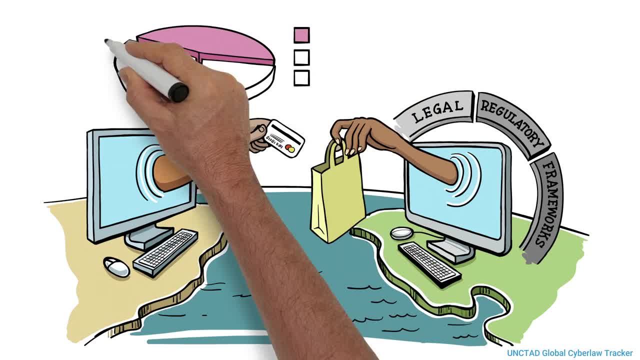 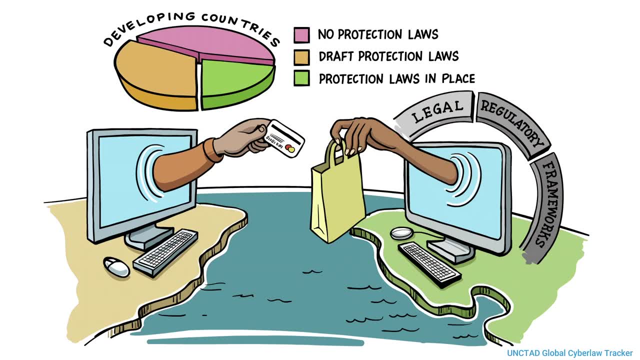 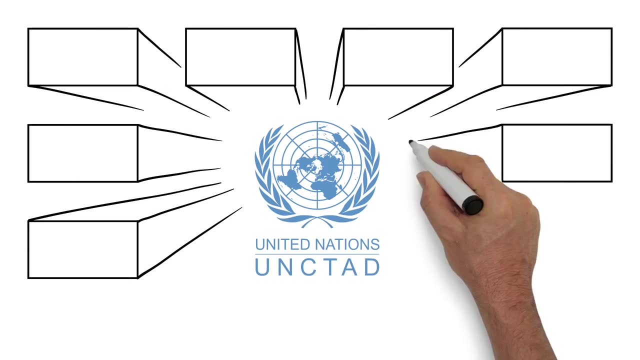 According to the UNCTAD Global Cyber Law Tracker, around 60 developing countries do not have current baseline protection laws in place and another 35 only have draft legislation. The United Nations Conference on Trade and Development is happy to offer a platform for discussion on a vitally important subject. 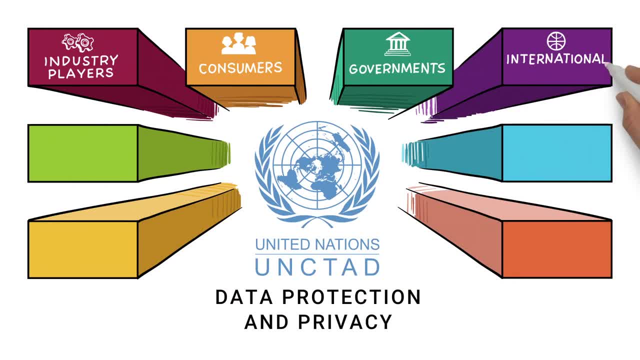 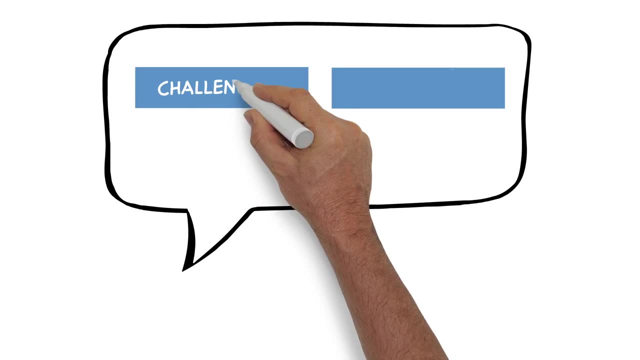 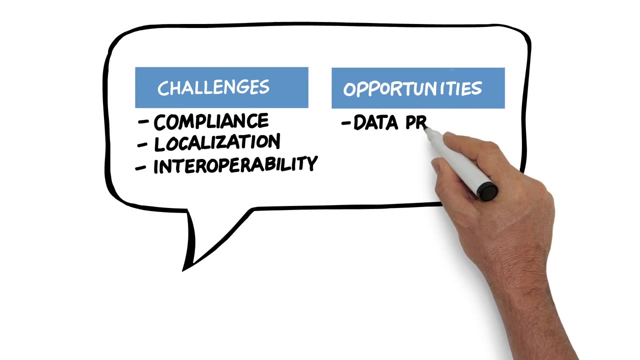 As industry players and consumers, as well as governments and international organizations. you will have the opportunity to present your perspectives, outline recent developments, current practices and consider relevant frameworks. We will discuss how various challenges, including compliance, localization and interoperability, as well as opportunities related to data protection and privacy, affect the potential for cross-border trade. 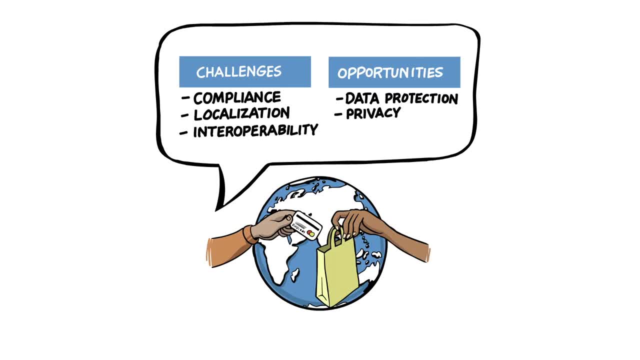 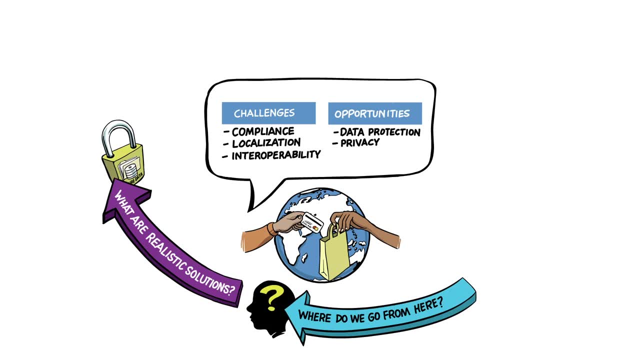 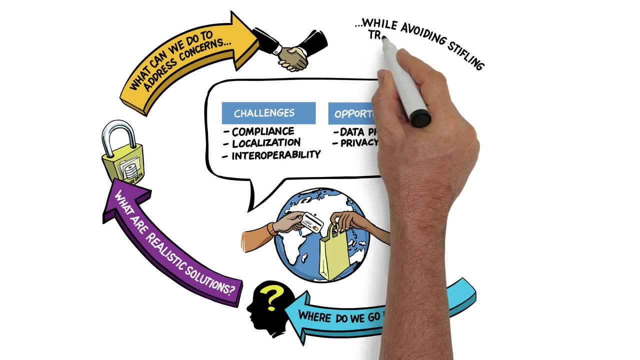 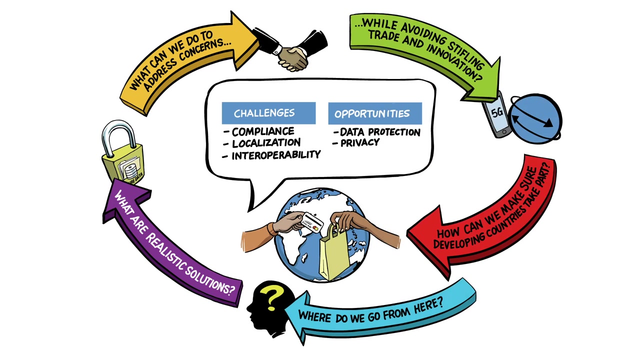 Especially in the context of developing countries. So let's start the dialogue. Where do we go from here? What are realistic solutions? What can we do to address concerns of various stakeholders while at the same time avoiding stifling trade and innovation? How can we make sure developing countries take full part in this global discussion and accelerate their adoption and enforcement of legal frameworks? 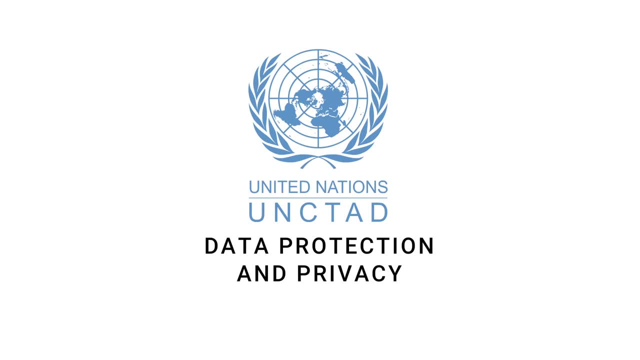 Welcome to UNCTAD and to the expert meeting on Data Protection and Privacy – Implications for Trade and Development.